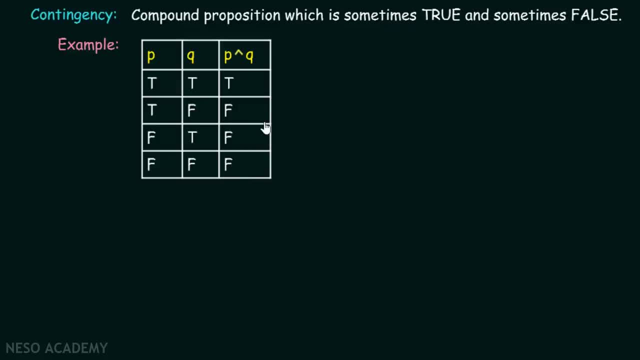 As we can clearly see from this truth table, And hence this compound preposition is a contingency. Okay, Now what is the meaning of satisfiability? A compound preposition is satisfiable if there is at least at least one true result in its truth table. 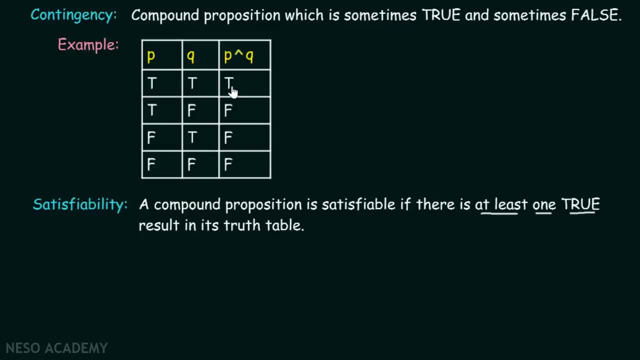 Simple: There must be at least one true result in its truth table. We can say that p and q is satisfiable because there is at least one true result in its truth table, Right. And we can also say that a tautology is always satisfiable. 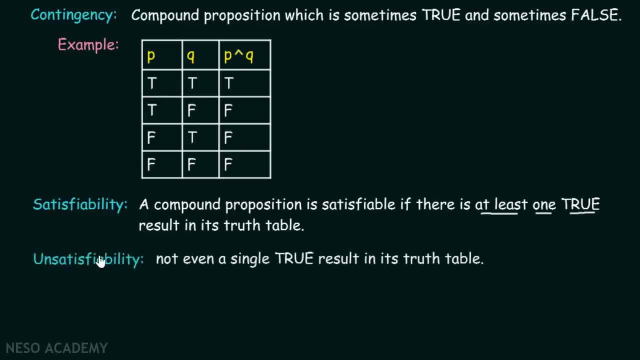 Isn't that so Let's try to understand what is unsatisfiability. Unsatisfiability means you will not be able to find even a single true result in the truth table of compound preposition. So we can say that a contradiction is always unsatisfiable. 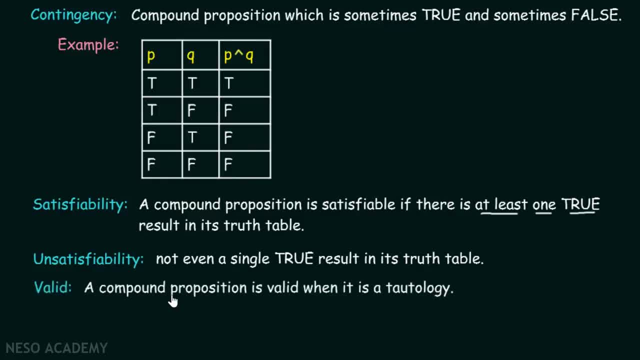 Right Now, what is valid? A compound preposition is valid when it is a tautology, And a compound preposition is invalid when it is either a contradiction or contingency. Now, this is a very important point to note: A compound preposition which is a tautology. 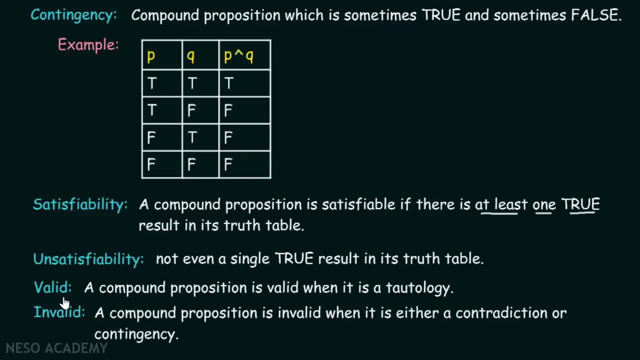 is always valid, While a compound preposition which is not a tautology is invalid. Not a tautology does not mean that it is always a contradiction. It can be contingency as well. Therefore, invalid covers both contradiction as well as contingency. 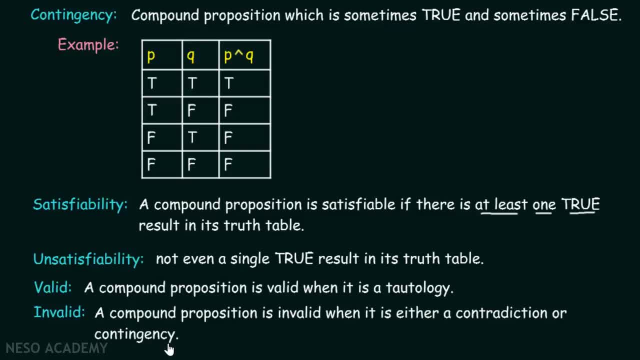 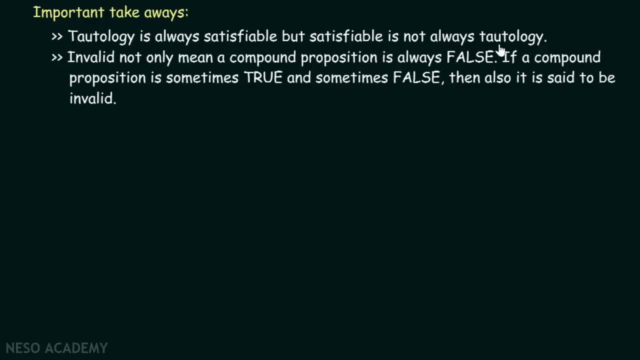 Okay, Now here are the takeaways for this lecture. Tautology is always satisfiable, but satisfiable is not always tautology. Please remember: we know that tautology is always satisfiable, But satisfiable is not always tautology. 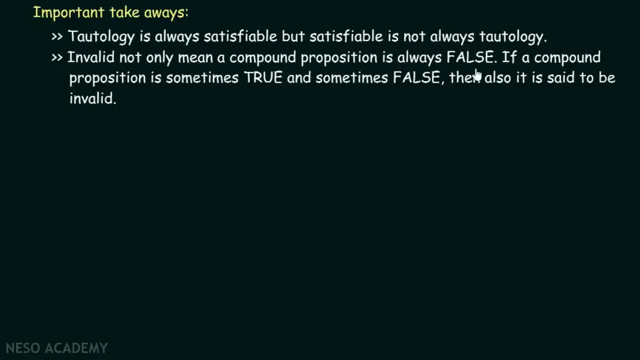 Invalid not only mean a compound preposition is always false. If a compound preposition is sometimes true and sometimes false, then also it is said to be invalid. We already know that invalid compound preposition is not always a contradiction, It can be a contingency as well. 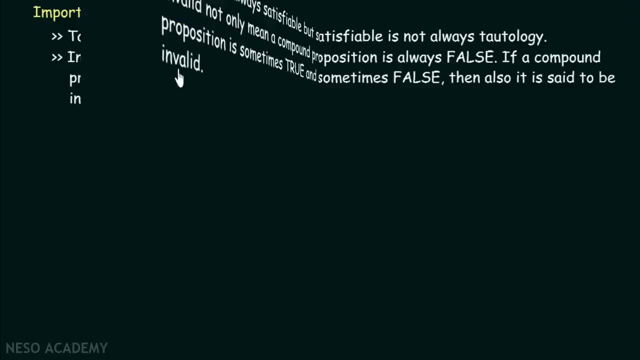 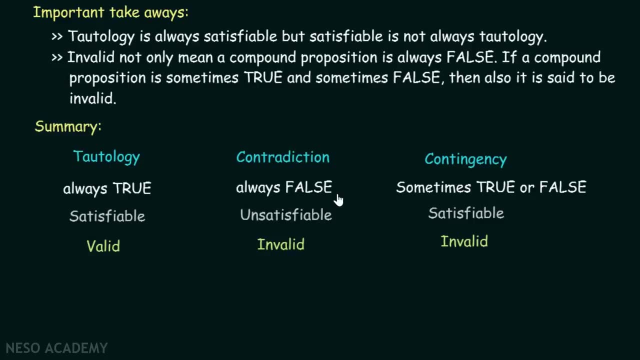 And that is what is being explained in this particular statement. Now here is the summary of this lecture. Tautology means always true. Contradiction means always false, Contingency means sometimes true or sometimes false. Now, tautology is always satisfiable.